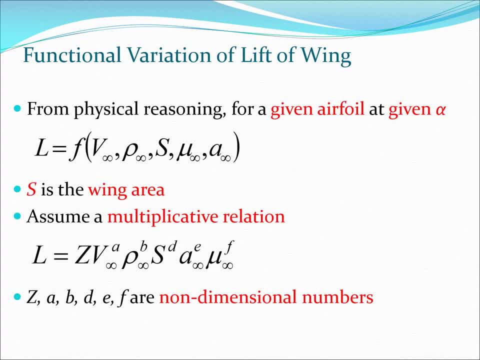 is concerned. So let us start with the mathematics. Now we know that the lift is going to be a measure or a function of several quantities. So these quantities would include velocity, density, the area of the wing, the viscosity, mu and the speed of sound, a. So these are essentially 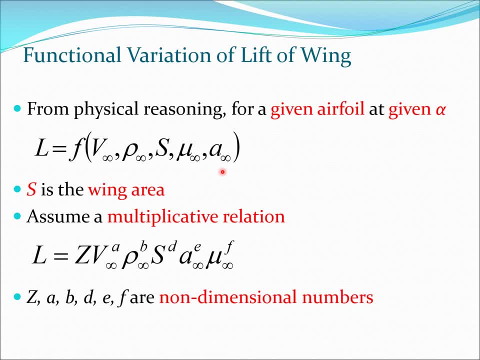 coming from our physical thinking about the situation. If you were to place any airfoil system in air, then you would naturally think that it is going to be a function of the density of air, the velocity at which the body is moving, the area of the body, and so on. So 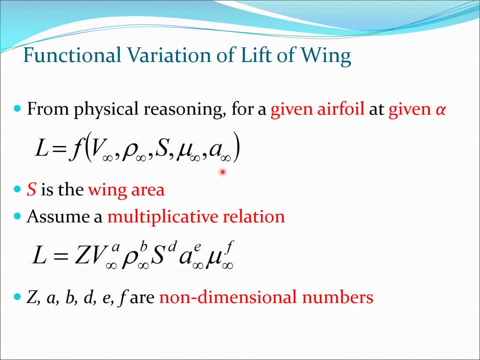 lift would be a function of these quantities and also from the fact we know about viscosity- because viscous flow is something which is a reality- and compressibility effects. typically, they would also be a function of mu and a, Depending on the speed at which you are flying, and so on. So we keep all these measures here and then. 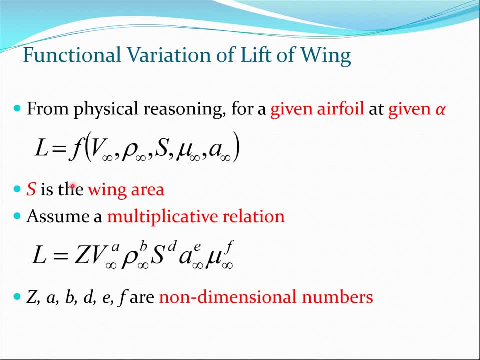 we will try to get the functional relationship, So L is a function of these quantities. Now, since we do not know this functional relationship, what we will assume as a very simple assumption is that it is a multiplicative relationship. So we say L is some value, z. 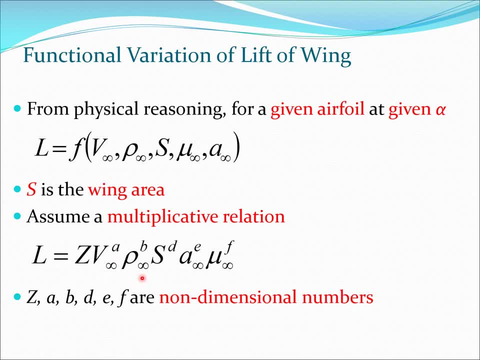 into v, infinity to the power a, rho infinity to the power b, s to the power d, a to the power e and mu to the power f. So here, all these values, z, a, b, d, e, f, are non-dimensional numbers. 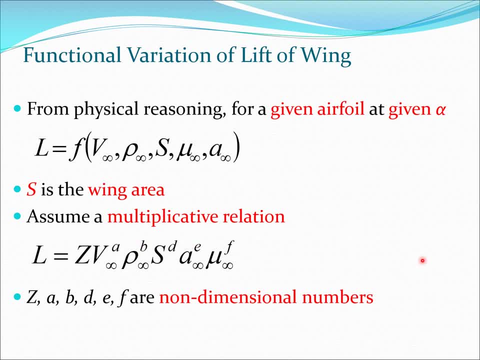 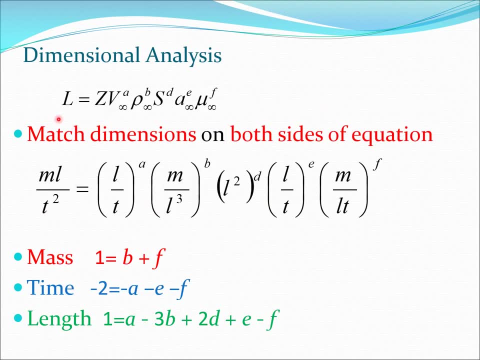 and we do not use the value c here because we already have kept c for chord. So we do not want any confusion about that Now. once we consider this to be our possible solution, then we will be able to get the functional relationship. So. 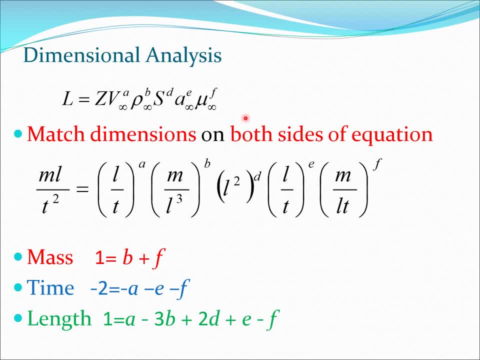 once we consider this to be our possible solution, then we will be able to get the functional relationship. So once we consider this to be our possible solution, then we will be able to get the functional relationship. What we are going to do is we are going to match the dimensions on both sides of this equation. 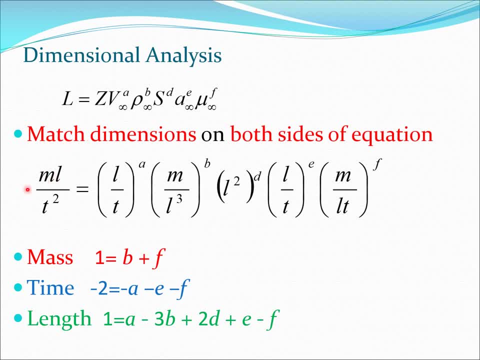 So, remember, the dimensions are expressed in terms of mass, time and length. So let us think in terms of unit. For example, lift is a force, So its unit is going to be in terms of Newton. or you could write it as: 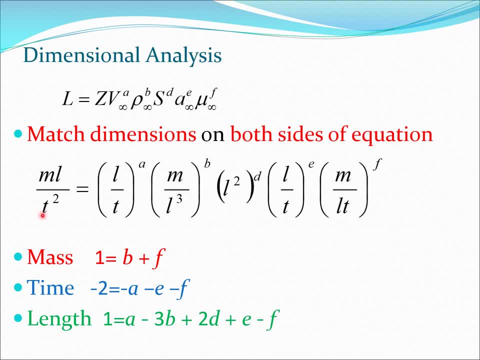 mass divided by t square into l, so this is the dimension of lift. similarly we see velocity is meter per second. so it's here. density is like kg per meter cube, then s is simply meter square, a is meter per second, again it's the speed of sound, and mu- we remember from the units of viscosity- is kg meter second. 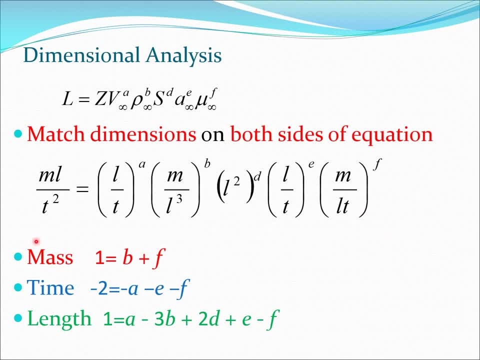 so, basically, from our knowledge of units of these quantities, we can easily write this relation out, and what this relation is going to help us do is that it's going to remove certain redundant indices which are there. so we are going to do that next. so what we do is now we write. 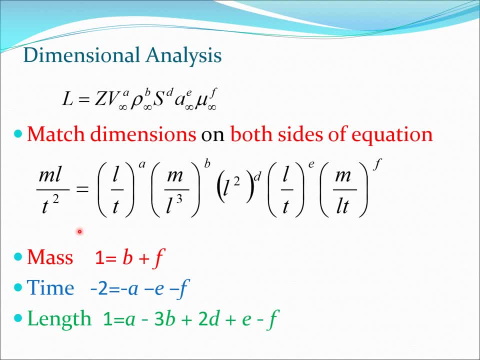 equations based on balancing the indices of each of these quantities. so let's look at mass first. so on the left hand side, mass has simply to the power one raised here, so it is one, and here mass has to the power b, so we have b plus f, so that's the second one, so one equals b plus f if we match the powers of m on. 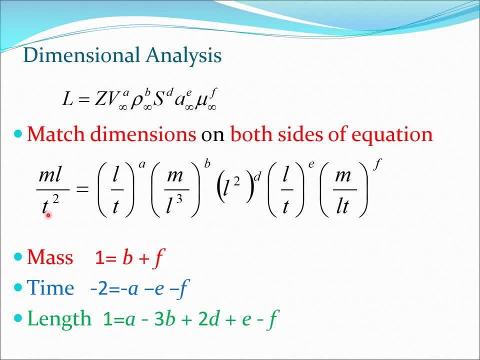 both sides similarly. we look at time. so time here is t, t, t. so it is minus two, because if we take the t up it becomes t to the power minus two. so that's the index here and here one index is minus a. then you have one more index is minus e and another index 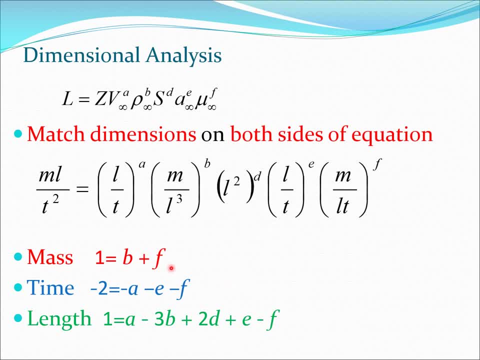 is minus f, so that comes in here. that's minus two, is minus a, minus e, minus f. now the third is about length. so here we take length. length has power one, so there's one here. it's power a, so that is a, and there is power minus three b, so that's here, so minus three b, because 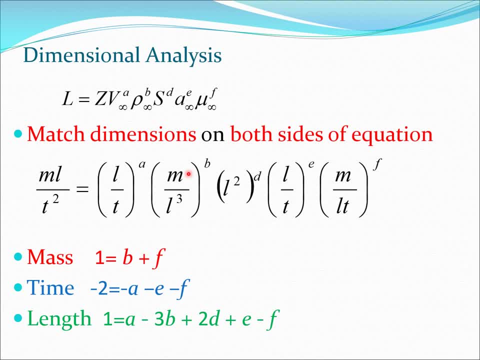 if we take l to top, it becomes l to the power minus three. and then we take the b, so it becomes minus three b. similarly two, d and l to the power e. so e comes here and l here is minus f, because l goes up, l minus one, and then f, so minus f here. so these three equations are going to help us. 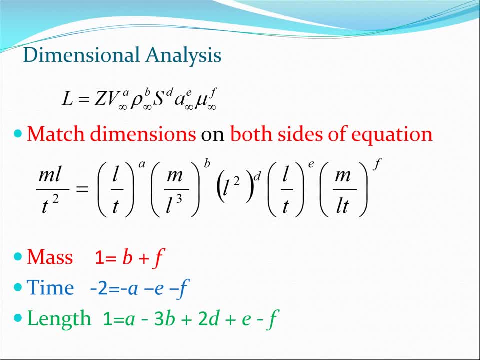 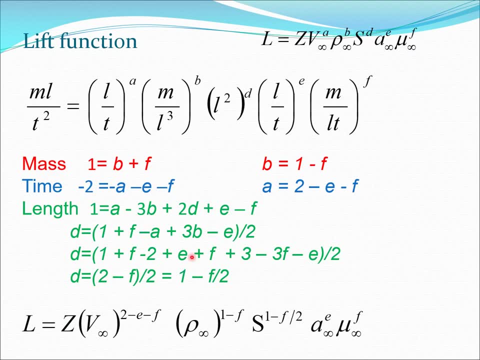 remove some of these quantities. so now, right now, we have a, b, d, e, f, so some are going to be removed. now, how we remove that is, we are going to simplify this. so, for example, if we have mass like this, i can write b in terms of f, so b would be 1 minus f. if i have time giving me this equation, then i can. 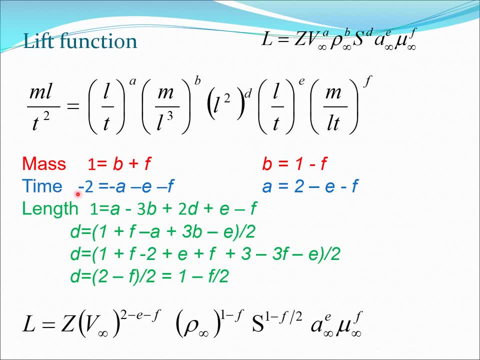 write a in terms of e and f, so a, if i take it to the left hand side, would be 2 minus e minus f, and then the third equation is going to give me the next quantity. but i have to do some math here, so let's start with the third equation here, and what i do here is that i substitute a and b from. 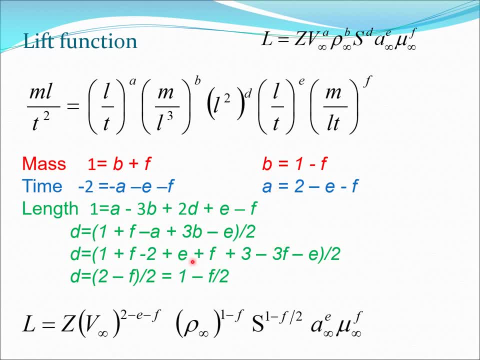 these two equations into the third equation. okay, so i substitute a is this value here? and so on on, and so that's going to simplify things for me. so first i write this d out. so i write: d is 1 minus f plus f minus a, and so on, so whole thing divided by 2. then i further expand this d out by: 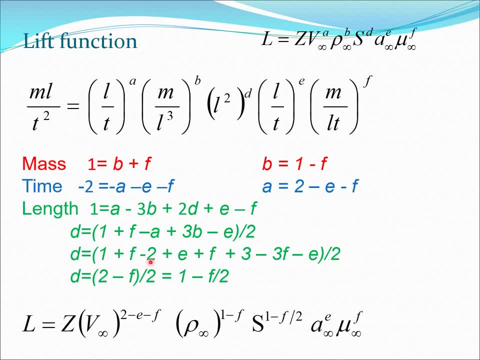 putting in the values for a and b, and then i get some cancellations, and the cancellations finally give me d is 1 minus f by 2. so essentially what i have done is i have got rid of a, b and d, and so i can write this l only in terms of e and f, which you see here. so now what we have is we have this: 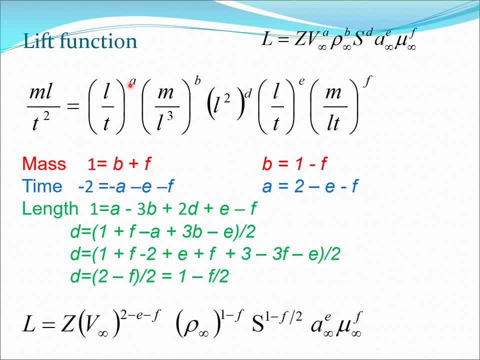 v, infinity, which was the velocity to the power a, and we know a is 2 minus e minus f. so we have that here, we have this, we have this and we have this, have the next one, which is density, and density had power b. so that's 1 minus f. 1 minus f comes here. 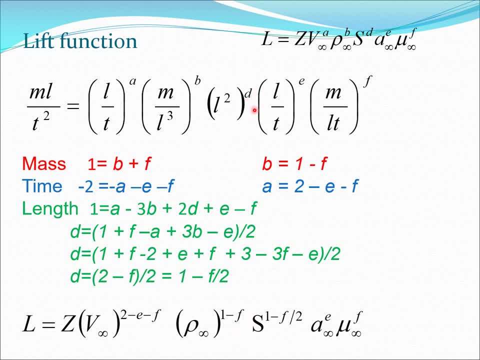 we had l square to the power d, so i have s to the power 1 minus f by 2, because d is 1 minus f by 2. and then i had the speed of sound to the power e and i had the viscosity to the power f. so this: 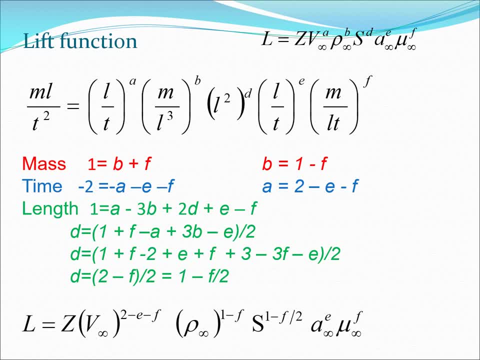 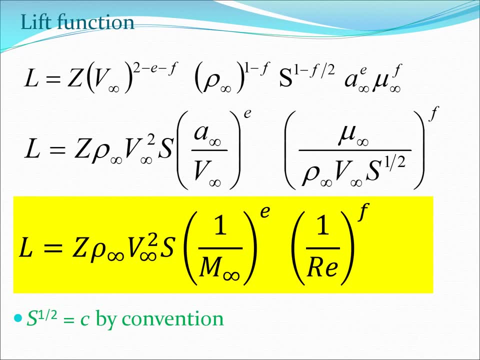 is now my new functional relationship of f, and so i have managed to remove some of the indices here. so now what i'm going to do is i'm going to take that equation which i wrote in the previous slide, and i'm going to simplify it further or write it in a different form. so let's say we pull out one. 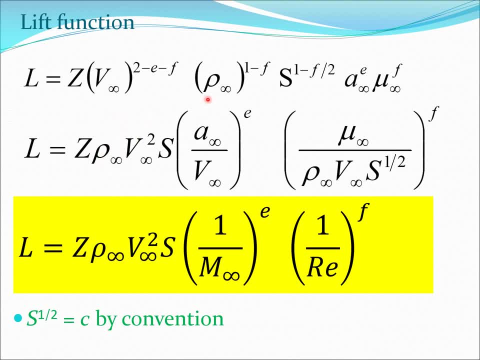 by one, the different quantities. so let's pull out rho infinity. here you see, there is a rho infinity to the power 1, so i can take from 0 to the power 1 and, if i can, rocks jewel, so i can take from 0 to the power 1. so i can filme the equation which i wrote in the previous slide and i'm going to 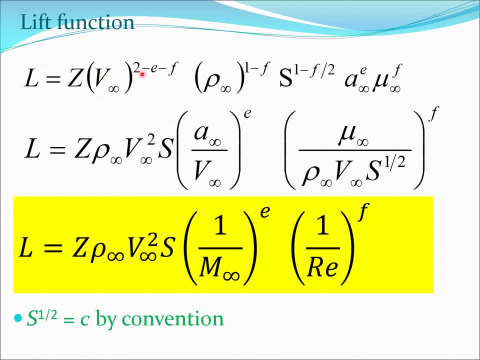 that out. here I get rho, infinity. there's a v infinity to the power 2, so that's this value here. and there is s to the power 1, so that's this value here. then I get a, and I get v to the power c to the power e, so I get a infinity or a infinity to the power e. that's this value. 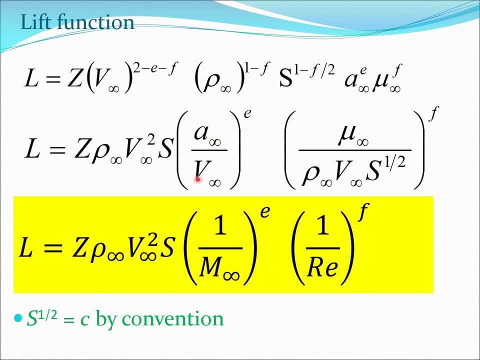 and then v infinity to the power minus e, so the v infinity goes down. and similarly I get mu infinity here, i get rho infinity minus f, which comes here, i get v infinity minus f, which comes here, and i get s minus f by 2, which comes here. so from this relationship i can immediately conclude: 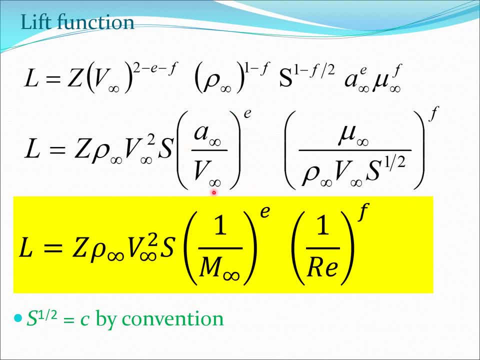 from my previous knowledge that this a infinity by v infinity is 1 by Mach number and this is 1 by Reynolds number, where we are using the fact that s half can be considered to be c by convention. so you clearly now see that the lift is a function of this particular value, which is 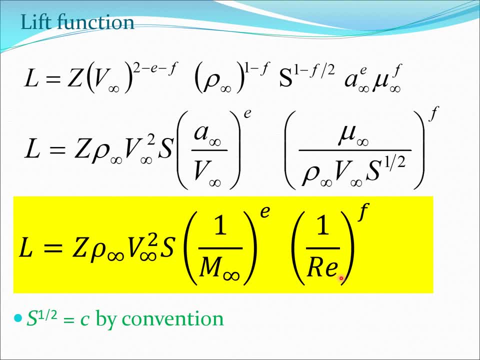 rho v s and then Mach number and Reynolds number. so this is a very important equation we have obtained. we now know that what we started with, the functional relationship, has led essentially to this relationship. so of course this also makes a lot of physical sense. we know that if we are flying an aircraft through air, it's going to depend on the density, because 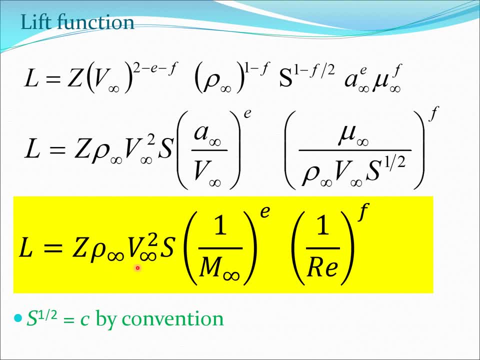 the density is going to produce the lift. it's also going to be related to velocity of the body and the size of the body, the size of the wing cord and so on, and also there is going to be some effect of Mach number and Reynolds number, because compressibility effects and viscous effects are. 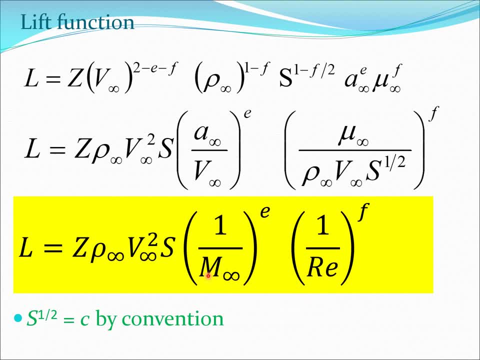 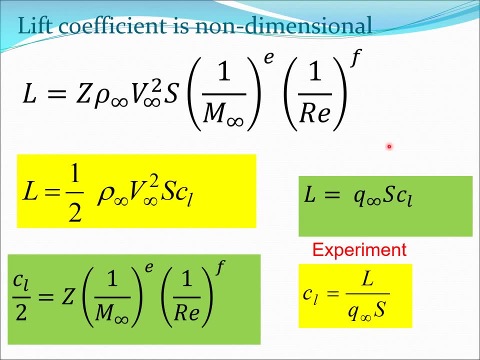 going to be important and these two effects are going to come in through these two numbers. so now let's write this formula again and let's now look at what we do to define the lift coefficient. so what we are going to do is we are going to write L as this form, so we are going to say L is. 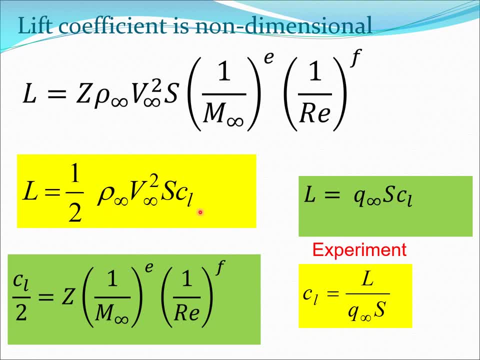 half rho, infinity v, infinity squared s, cl. and to do that I have to define cl in this form. so essentially, cl is used to absorb all the remaining coefficient of ellipses and so on and so forth. so here, and if you take a good look you can clearly see this is non-dimensional, because mark number 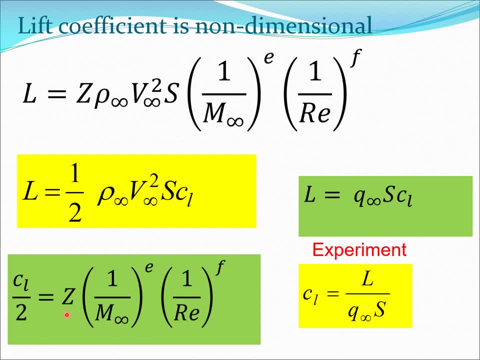 reynolds number were both non-dimensional and we also had assumed z is non-dimensional and of course e and f are non-dimensional numbers. so this is the value of cl here. now, from this equation you we cannot just calculate cl because first of all we do not know what is z. we do not know what. 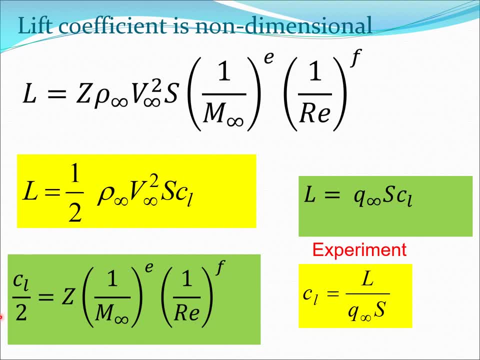 is e and f and so on. but we know that there is some value here, some lift coefficient which would be expressed in this form. and if i write this equation here, which is essentially same as l is dynamic pressure into the area, into cl, then i can write: cl is l by q, infinity s, so this gives me a. 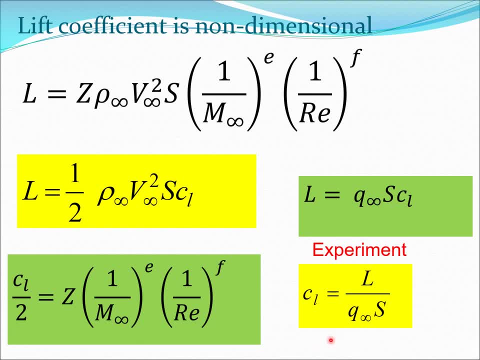 way to calculate the lift coefficient. so essentially, lift coefficient could be calculated, for example, by experiment. if i were to take a certain wing or aircraft and put it in a wind tunnel, i could get a lift. i could measure that. i could calculate q infinity because i know half rho v square, i know the density of air. 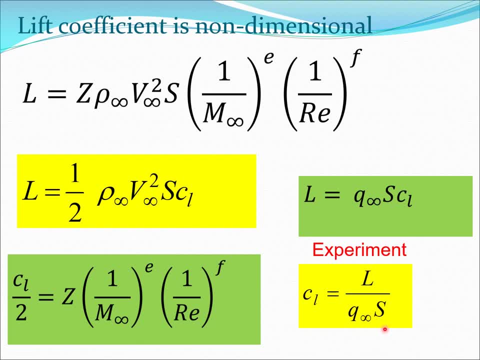 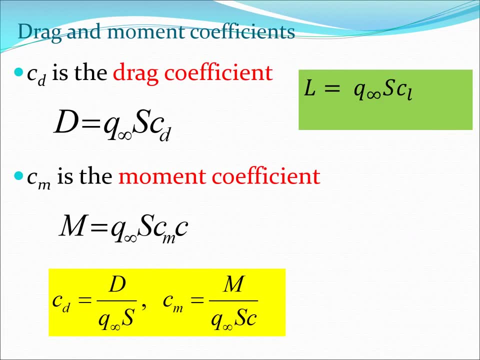 i know the velocity of air and i also have s from the geometry of the body, so essentially i could calculate cl from experiment. now the same kind of thought process can be used to get the drag coefficient, that is cd, and the moment coefficient, that is cm. so, for example, if i were to write the drag, the drag, 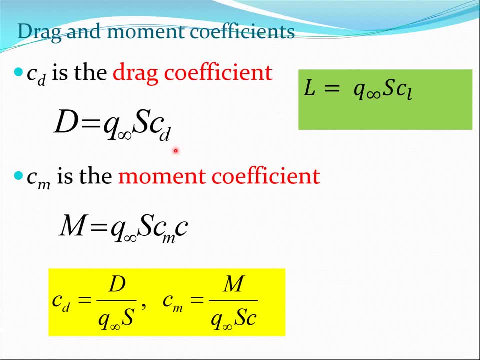 would come out as q, infinity as cd. so you exactly follow that same dimensional analysis process and you will get this equation. and also you will get moment is q, infinity as cmc. and this extra c comes in because we are talking about moment here, so it is a force into a distance. so that gives me the 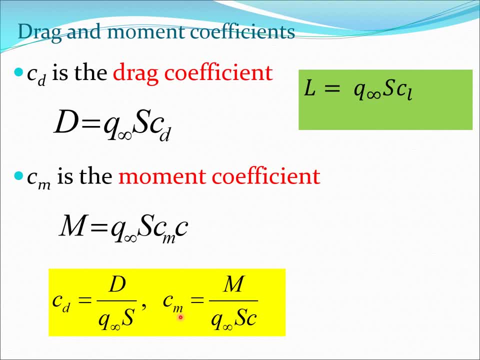 moment. so again, if i were to write the drag coefficient, that is cd, and the moment coefficient, i wanted to find cd and cm. i could do it by experiment because they are related to the measured drag and the measured moment and of course i would have chord also. that's a geometric 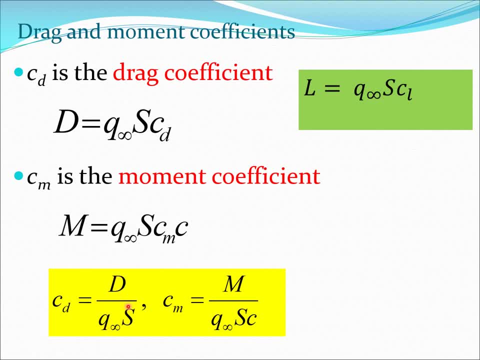 property of the system. so in these equations we essentially have the lift, drag and moment, which are measurable properties of the system. you have q- infinity, which comes from density and velocity, which are coming from properties of the air, and then you have s and c, which are geometric properties of the system, which are essentially the properties of the aircraft or 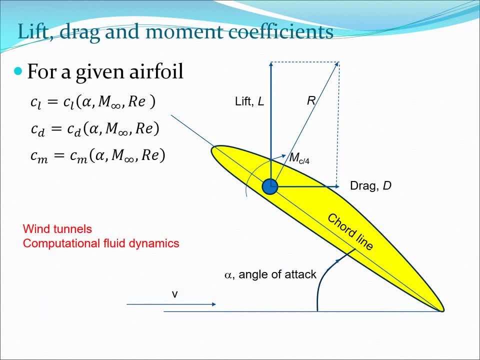 whatever flight vehicle you are working with. so now we again go back to our figure of the airfoil section, which was discussed before and now we have, for a given airfoil, cl is a function of alpha mach number and reynold number, cd is a function of alpha mach number and reynold number, and cm is a. 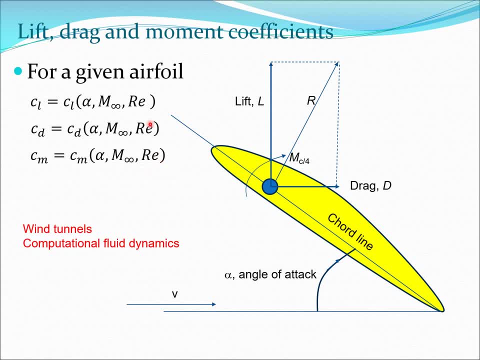 function of alpha, Mach number and Reynolds number. So if we keep these Mach number and Reynolds number fixed, then if we vary alpha we can actually get C L. is C L alpha, and later we are going to see that we can plot some of those figures and so on. Now how you would. 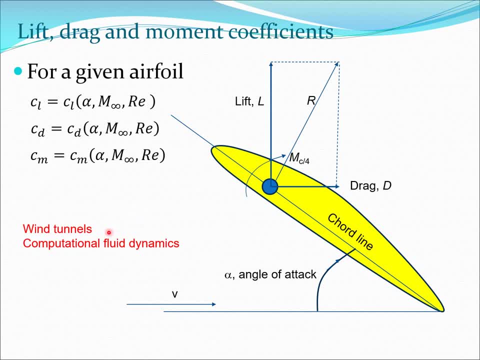 get these values C, L, C, D and C, M. So again, lot of people did experiments many years ago and they are all tabulated. There is a book on wing sections, I think by Ebert and Fondonoff, and you can look at the book for all the different tabulations, For example, for NACA 0012, airfoil. 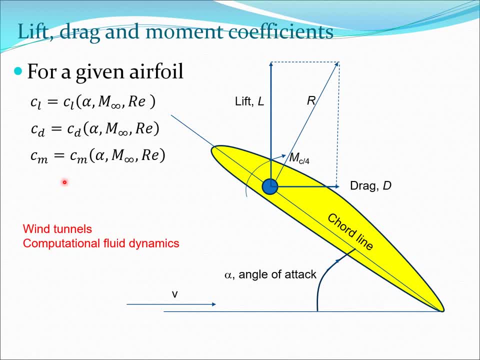 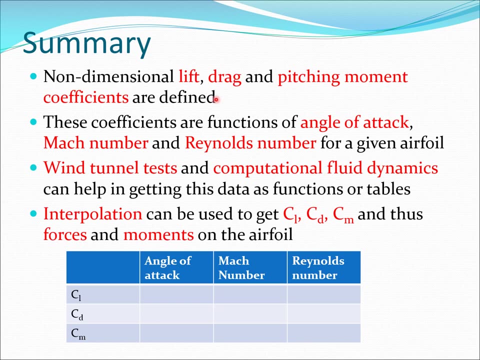 if you go and look there, you will find various tables for that, and also you could get it from some of the modern tools such as computational fluid dynamics and so on. So let us summarize today's class. We saw that there are non-dimensional measures of lift, drag and pitching moment, and these are the coefficients related to. 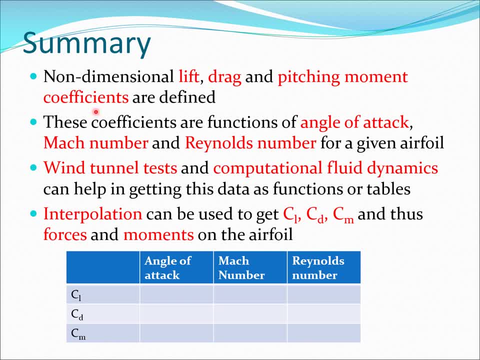 each of these forces and moments and we defined these coefficients. We use some dimensional analysis techniques to get there. We also saw that these coefficients C, L, C, D and C- M are functions of alpha Mach number and Reynolds number for a given airfoil and wind tunnel. 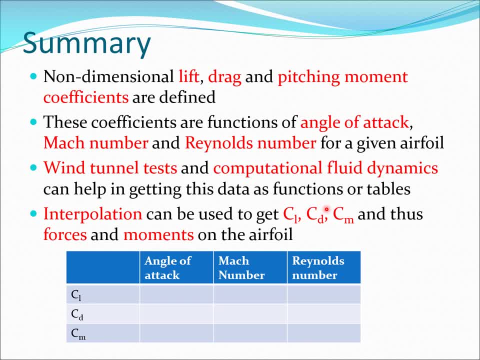 test and computational fluid dynamics can be used to get all these data as functions or tables, And these are essentially obtained at a variety of points, and then, if you are at a particular point in terms of alpha Reynolds number and Mach number, we can use numerical interpolation. 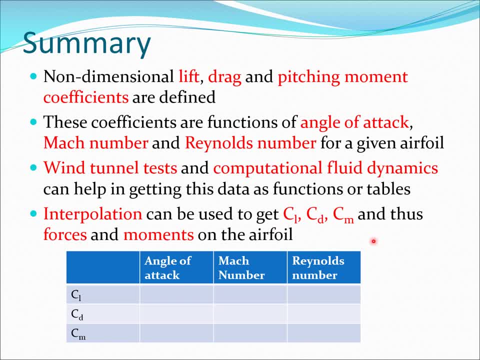 to get the precise values of C, L, C, D and C M. and once we have C, L, C, D and C M, we can calculate the forces and moments on the airfoil or the wing section. So do remember that if I have C, L, C, D, C M, then if I can get the dynamic pressure, 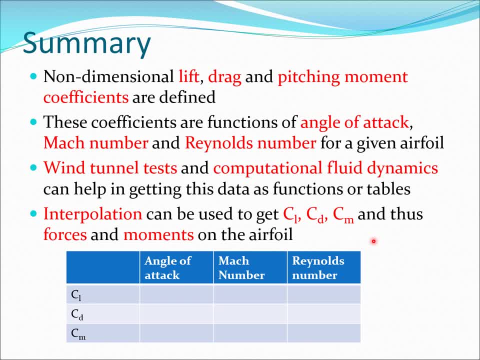 I can get the wing area of the chord and so on. I can very easily calculate the forces and moments. So in many cases you have this data available in tables like this. So here I have mentioned C, L, C, D, C, M, you have different angles, you have Mach numbers and 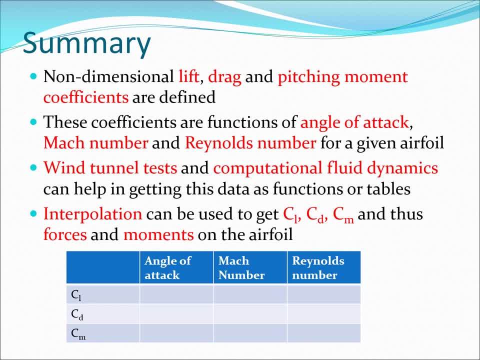 Reynolds numbers, and so if you have ever taken a numerical analysis class, you know there are interpolation techniques which can easily be used to find precisely at the alpha. you are at, At the M, you are at, at the Reynolds number, you are at what is the value of C, L, C, D? 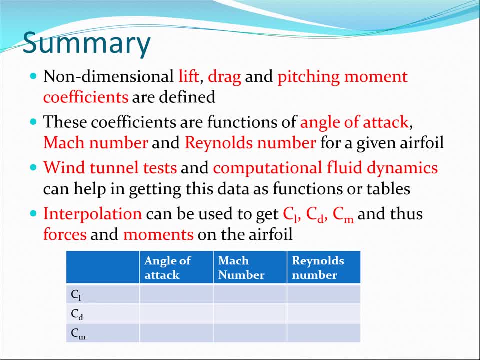 and C, M, and this is often used in many computer programs which are written to generate the values of lift, drag and pitching moment, which are further used to calculate the aerodynamic loads which act on the aircraft, which again then, are fed to the structural loading of 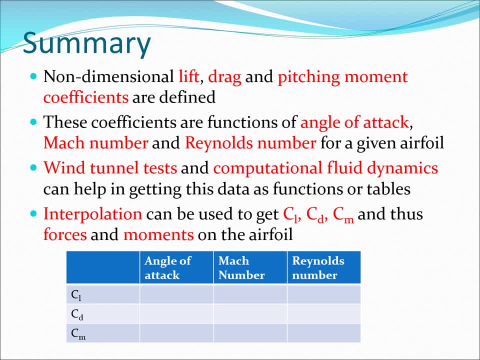 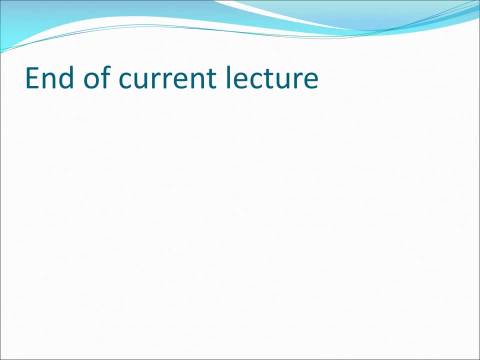 the system or for performance or flight mechanics purposes. So this was a lecture for today. this is an important lecture Because you clearly saw how the C, L, C, D and C M can be obtained and how it is actually a very good use of the dimensional concept. So I hope you enjoyed this video. I will see you in a video sometime soon. See you then.